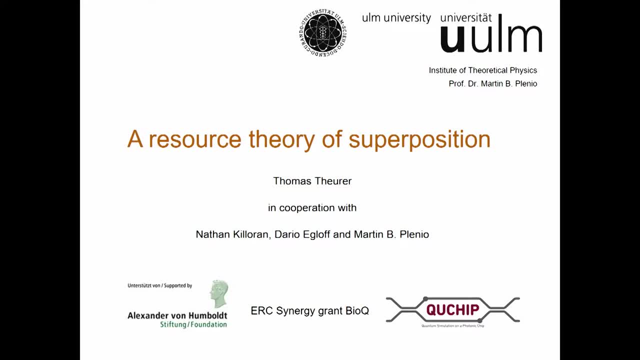 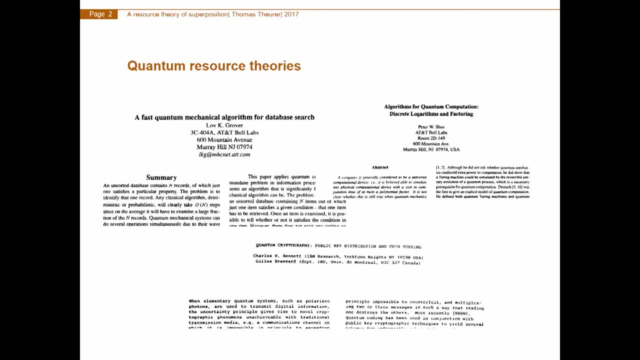 with Nathan Killoran, Dario Egloff and Martin Plenio. So let me start with a few words concerning quantum resource theories in general. Well, as you all know, there are protocols and devices which work on the laws of quantum mechanics that outperform their classical counterparts. 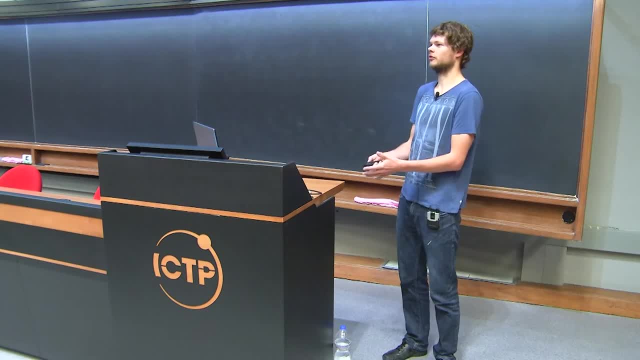 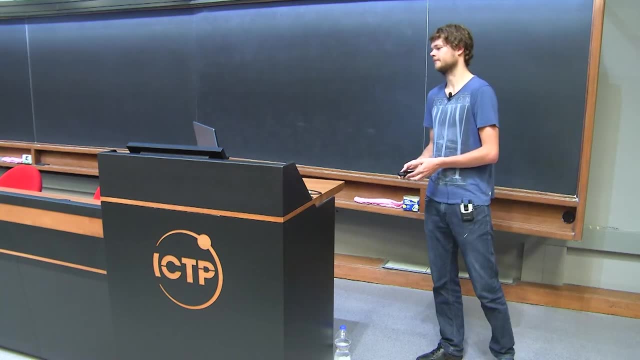 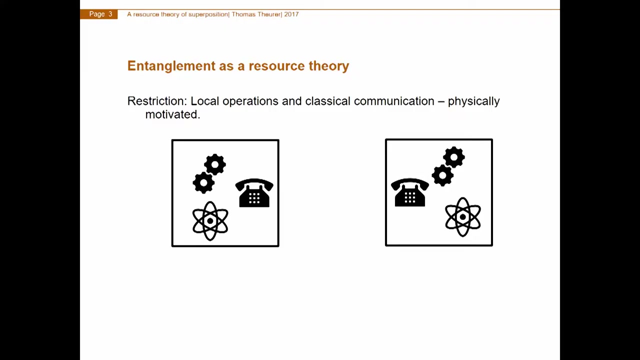 Now a natural question is why? What in quantum mechanics makes this protocol more efficient than classical protocols? And one way to attack this question is in the framework of resource theories. So the most studied and most established quantum resource theory is entanglement theory. 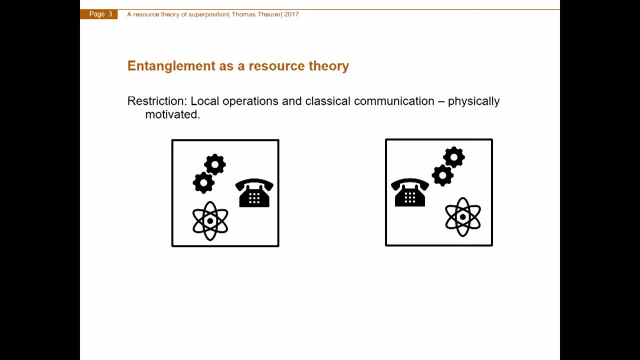 and it's based on a restriction. All quantum resource theories are built on a restriction that is placed on top of the laws of quantum mechanics. In this case, of entanglement theory, the restriction is the restriction to local operations and classical communication, and 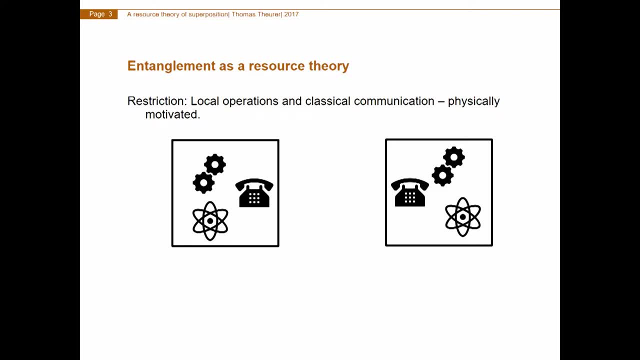 that is a physically motivated restriction, because it's much easier to communicate classically, because you can amplify classical information but you cannot amplify quantum information in general. So then, with this restriction, the property on a study is entanglement, because it cannot be created using only local operations and classical communication, but it allows. 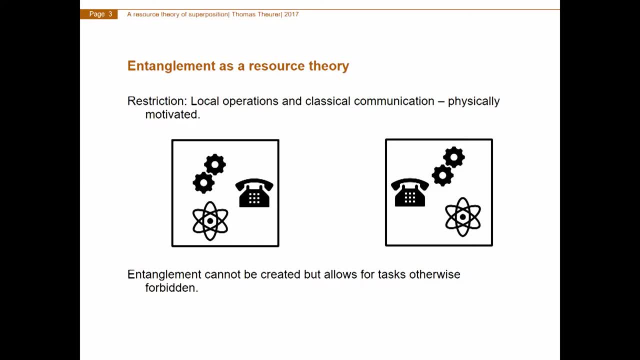 for tasks. The restrictions are also limited to the other things which are forbidden otherwise. For example, it allows one to overcome the restriction. The simple example would be: I teleport my system from one lab to the other lab, then I do whatever I want and I teleport it back. 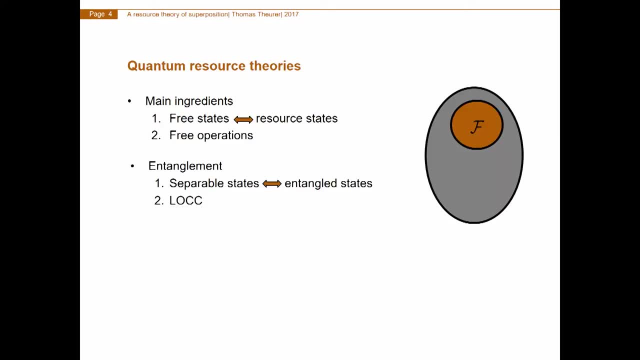 So I've. with the use of entanglement. I've overcome the restriction to local operations. Now, in general, all quantum resource theories are built like this. One puts in an additional restriction which should be modified physically. emerge two main ingredients. 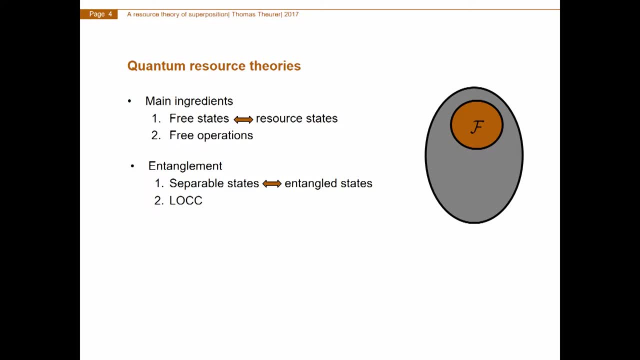 The first one is the free states, So these are the states that are easy to create or simple, And the second ingredient are the free operations, And the minimal restriction onto the free operations is that at least they should transform the free states into free states. 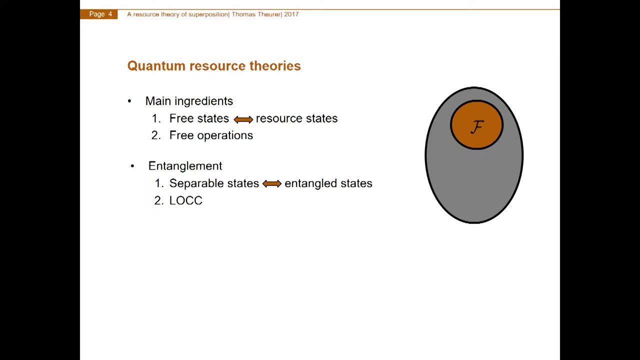 Otherwise they could create resources for free. Now, in the example of entanglement theory, these are the separable states and LOCC, And then all states that are not free. we call them resource states. Now, once this basic framework is set, one tries to answer. 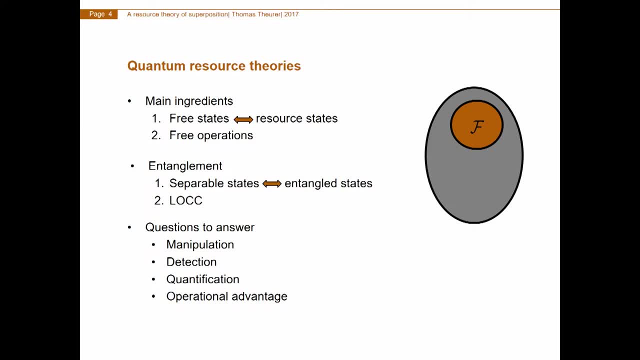 questions like: how can I manipulate my resource, So can I transform one resource state into another one using only the free operations. How can I detect a resource, both theoretically and in the lab, with measurements, And how can I quantify the resource, So can I introduce an order or a partial order into the. 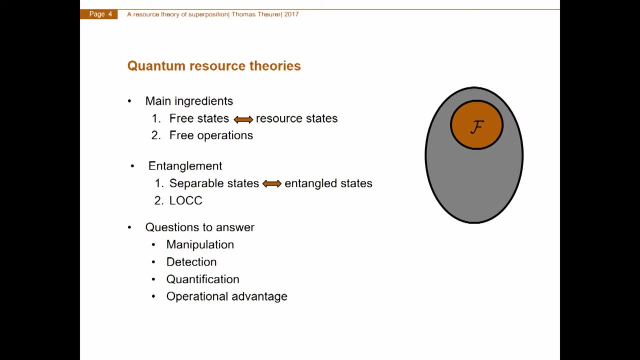 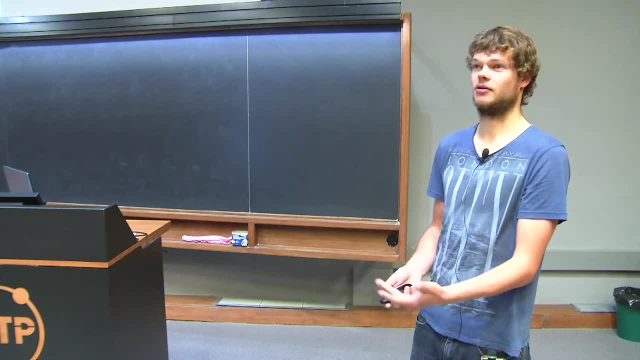 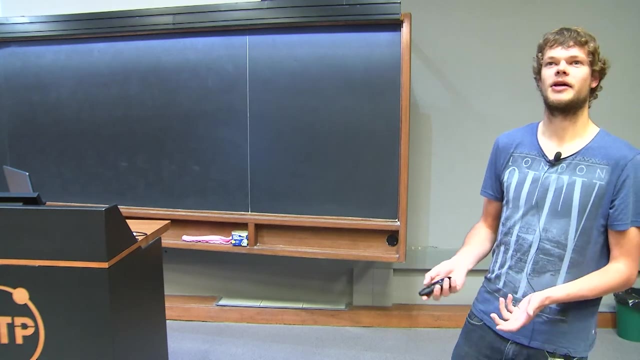 resource states. And all this is in mind, usually with operational advantages. So one wants to use the resource in order to perform some tasks better than without the resource. And in addition- so that's basically the idea for applications- it helps to study the property by itself from a. 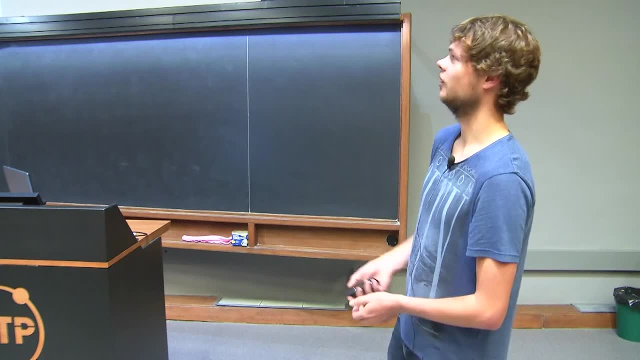 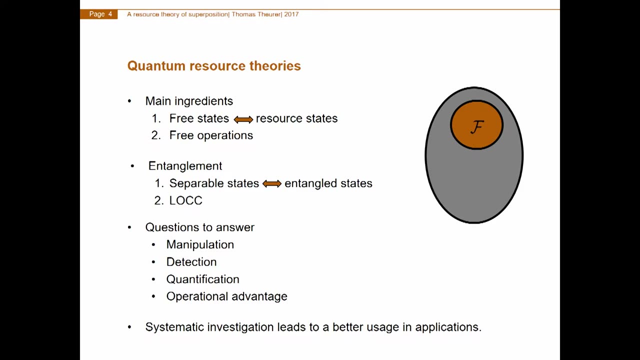 fundamental point of view. Now, if one investigates these questions rigorously, then one hopefully understands the resource better and so one can use it more effectively. Fighting these oswe day are hopefully been sufficient in new applications, or one even finds out which. 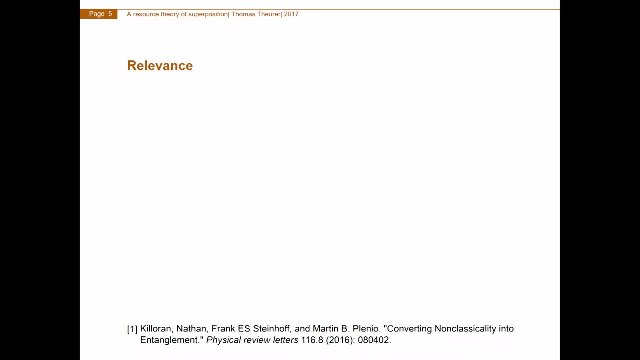 resource is present. in which application? Now let me modify the resource theory I will present to you now. So, in principle, all properties of quantum mechanics that you cannot reproduce using classical physics can lead to an operational advantage. So, in general, all types of nonclassicality are. 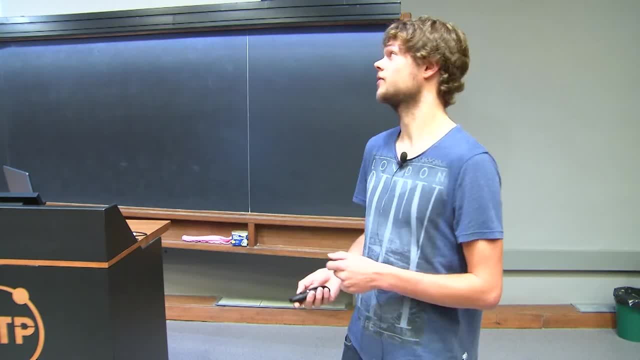 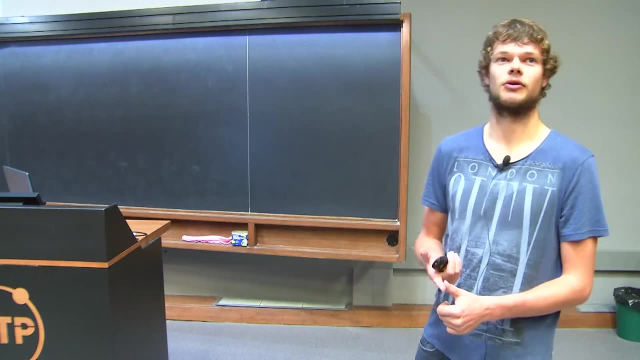 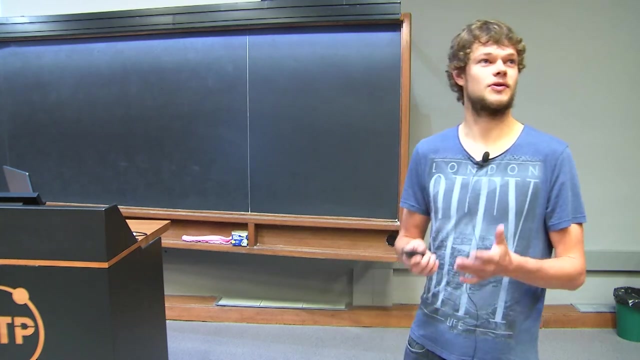 عf+ a resource, or might at least be a resource. One underlying principle of different quantum properties is the superposition principle. So in coherent theory one studies the superposition of orthogonal basis states. In entanglement theory one studies the superposition. 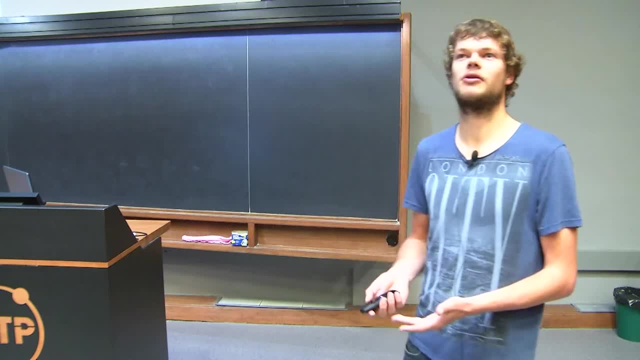 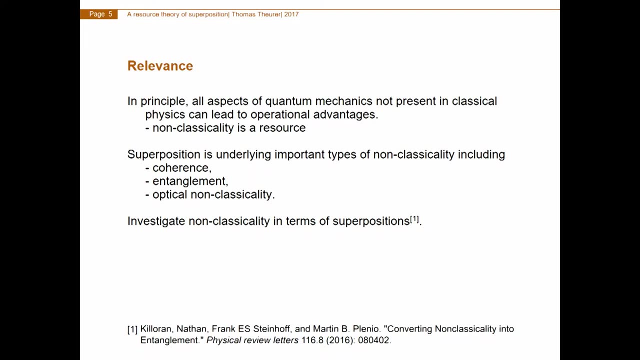 of separable states and an optic well, basically, optical non-classicality is the superposition of global, coherent states Now, so it's very natural to investigate non-classicality in terms of superpositions, and that's exactly what was done in this paper here. 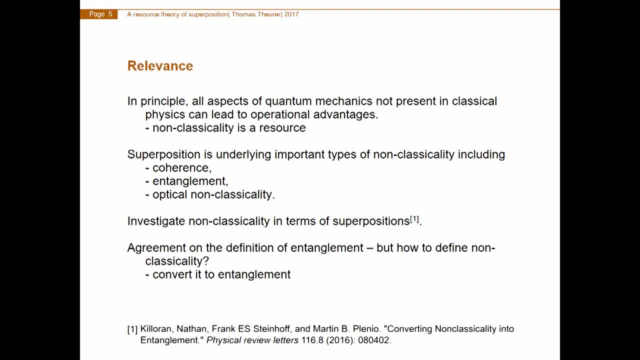 Now, if we want to define entanglement, there's a relatively big agreement on how we do this. But non-classicality in general is not a very well-defined quantity. So one idea to quantify non-classicality like mathematically rigorous is: can we convert it to entanglement. So if you can convert a state to entanglement, an entangled state using a fixed operation, then it's a non-classical one. If we can't, then it's a classical one. 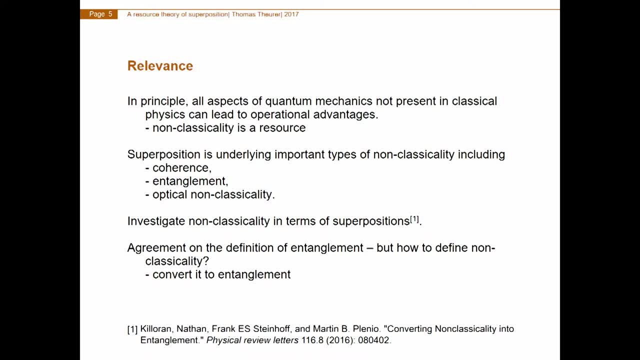 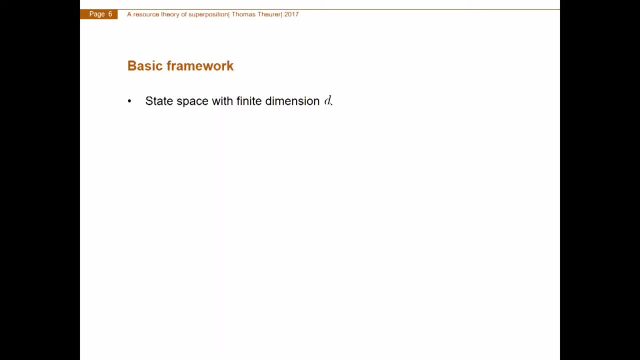 And with the theory I will present you here, that's exactly possible. So we can use the theory to define non-classicality via entanglement. Now let me come to the basic framework, or the mathematical framework I will use. First. we only consider finite dimensional Hilbert spaces. 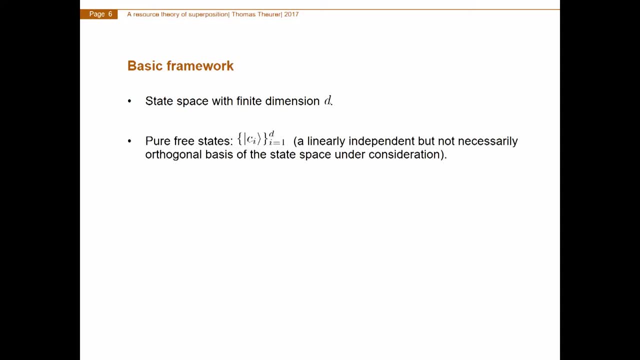 or state spaces. And the pure free states are defined by these CIs. And these CIs they form a linearly independent but not necessarily orthogonal basis of the state space under consideration. So in coherence theory, these pure free states, they are orthogonal. 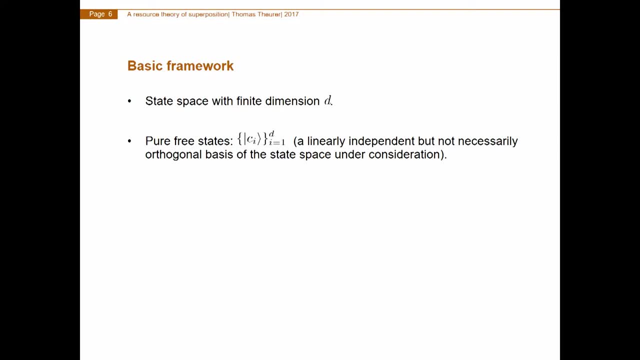 here not, And I will tell you later why we made this choice. Now, the free states in general are just statistical mixtures of pure free states And the free operations they are defined using free cross-operators, the cross-operators KN. here. 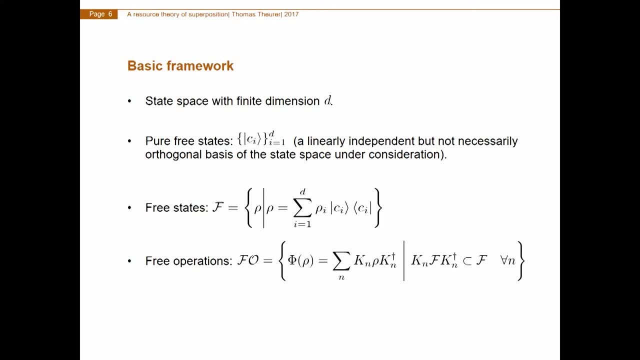 And they are constructed in a way that they map the set of free states into itself. Now then the free operations in general. they are all quantum operations that can be decomposed into these free cross-operators, and they should be trace-preserving. 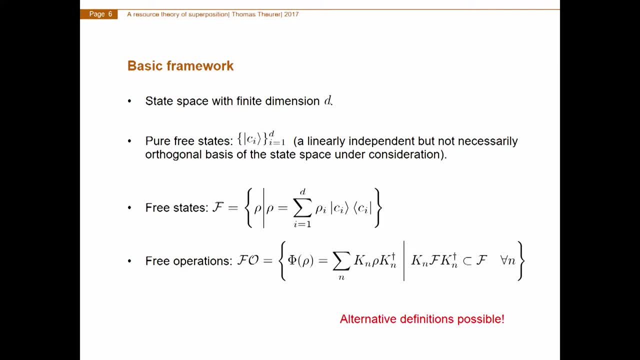 Now, as in coherence theory or in most other resource theories, you can define other sets of free operations and this gives rise to other resource theories. So that's not a special feature of this resource theory and it's not a deficit. 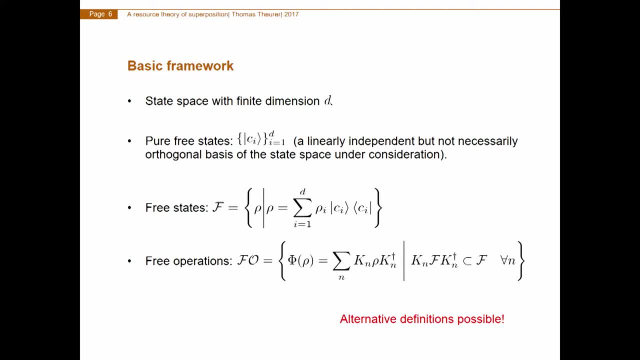 For example, in entanglement theory one could also consider only one-way classical communication, and that's for some application a well-defined setting which gives rise to another resource theory, but to a meaningful resource theory nevertheless. So I will not comment on alternative definitions. 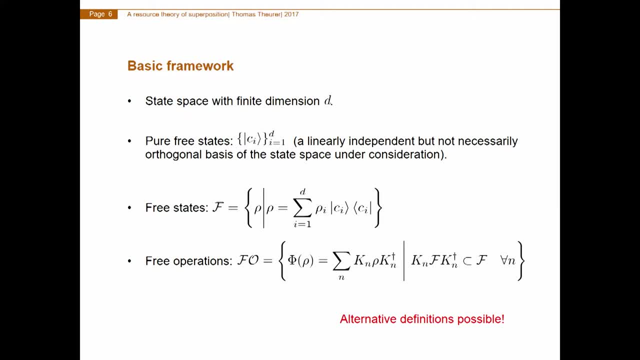 of the free operations. I will just say why this one is a good one, basically. So if we see this quantum operation as a generalized measurement with outcomes N that are associated with these cross-operators KN, then if we are allowed to sub-select, 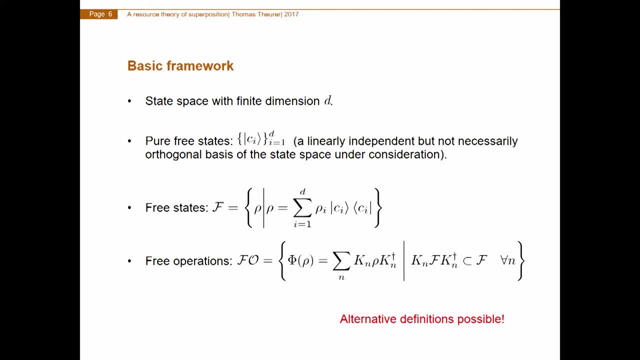 according to this measurement outcomes, we can never deduce that resource states have been created out of free states. So, in a sense, this is the maximum set of free operations. That is the maximum set of free operations. So, in a sense, this is the maximum set of free operations. 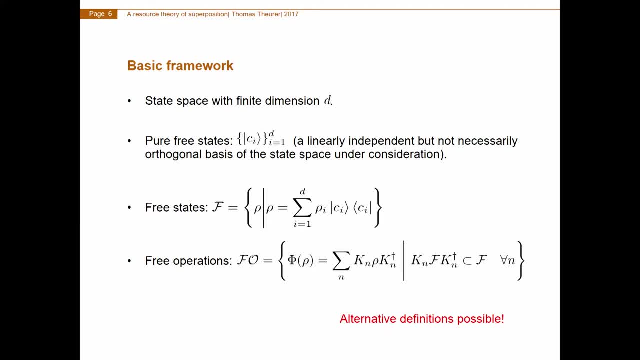 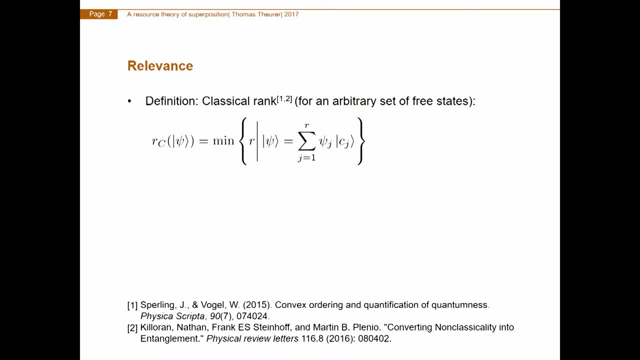 That is the maximum set of free operations And that, if we are allowed to do post-selection, cannot create the resource for free. Now let me come back to the relevance of this theory. So if you want to define non-classicality, 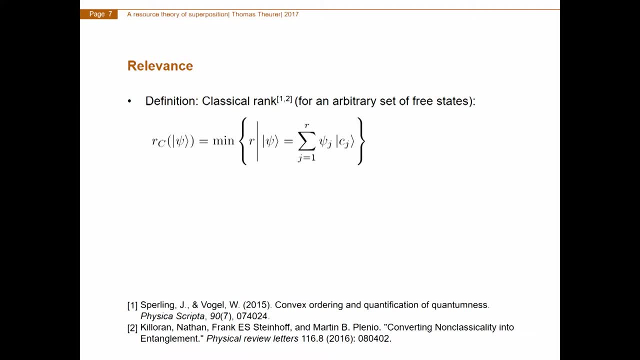 using the principle of superposition, then you can use what is called a classical rank, and it has been introduced in these two papers. So if we have a general set of free states, so in this case not linearly independent. 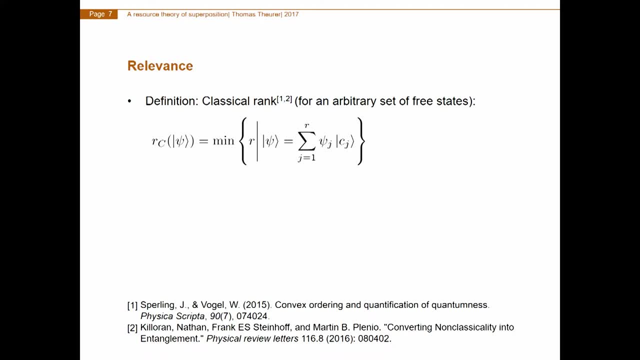 then the classical rank of a pure state is just the minimum number of free states we have to bring into a superposition in order to represent the state. So in a sense this is the analog of the Schmitt rank in bipartite entanglement. 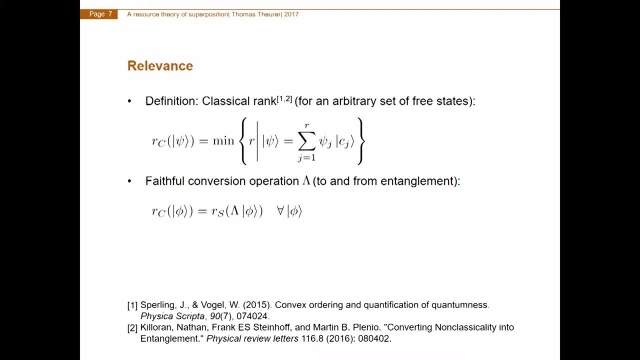 And now, having this quantity, this classical rank, we can define a faithful conversion operation. So this is a physical operation That transforms all pure states with a given classical rank into an entangled state with the same Schmitt rank. The idea behind this is that 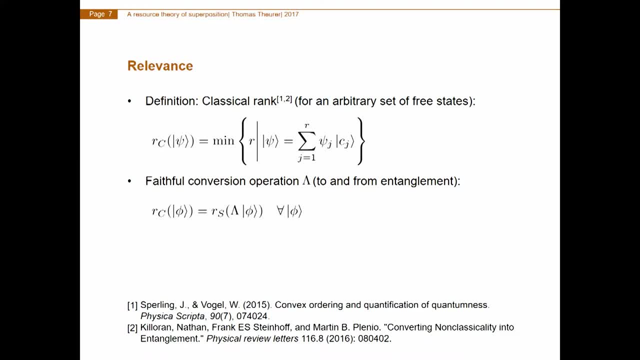 we do not create entanglement out of nothing, but we rather transform the resource of non-classicality into the resource of entanglement. Now, these faithful conversions, they allow for the definition of non-classicality because we can just say now: 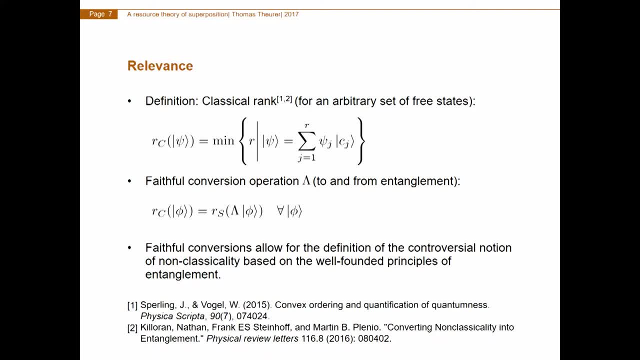 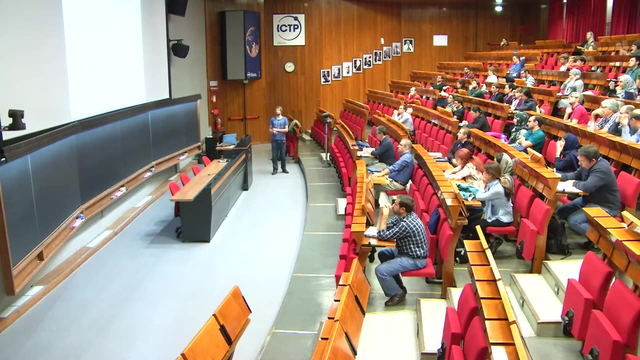 we quantify the state of non-classicality. We quantify the amount of non-classicality by the amount of entanglement we can create using this fixed conversion operation. RS is the Schmitt rank, Now not for all set of free states. 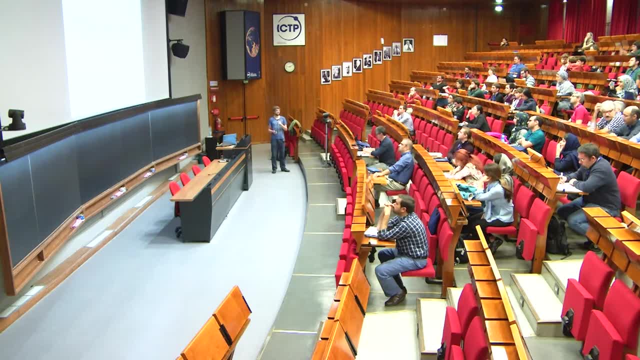 such faithful conversions exist, And indeed such faithful conversions if you are in a finite dimensional Hilbert space and have a countable set of free states. they exist if and only if the free states, the pure free states, are linearly independent. 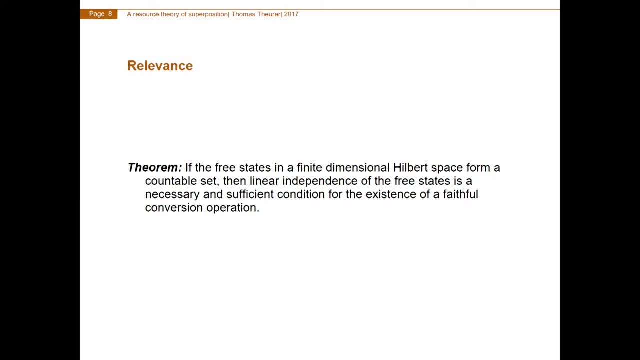 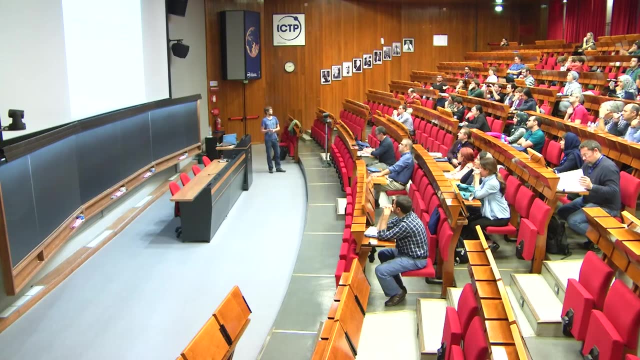 So that's why I made at the beginning a choice of linear, independent, free states. Now these faithful conversions. we will see later what an example for these conversions is. So in addition, the theory here is a generalization of coherent theory. 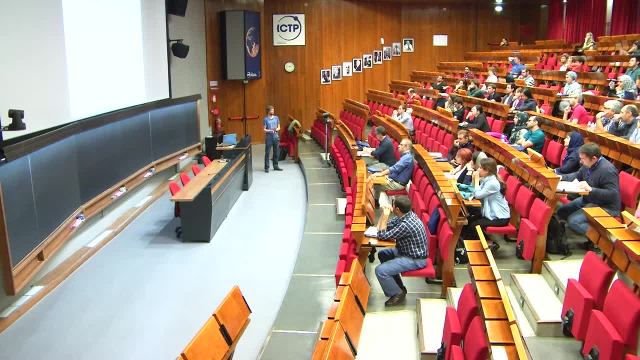 So coherent theory is the same theory where the free states are orthogonal And in a sense, this allows us, from a conceptual point of view, to study the importance of orthogonality versus linear independence in such theories. Well, now for a precise example. 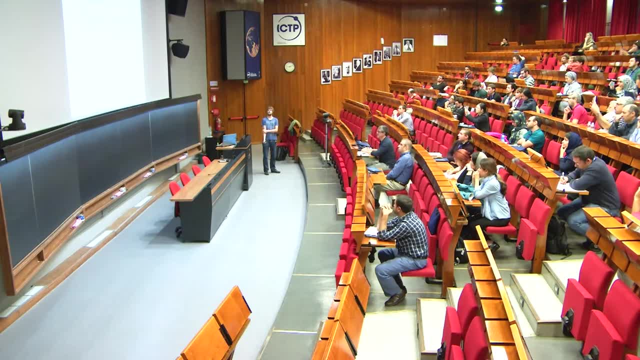 where we can use this theory is in quantum optical non-classicality. So if we have a finite number of global coherent states, then we can use this theory to study the non-classicality in their superpositions, Because a finite set of 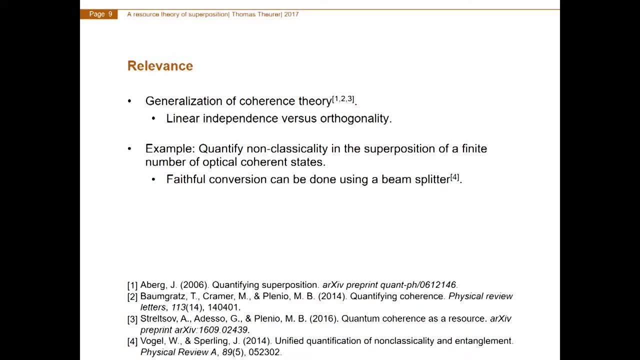 optical coherent states is linearly independent, but they are not orthogonal And in this case the faithful conversion operation can be done using a simple beam splitter where the second input port is in vacuum. So this would be a conversion operation which is really easy to implement in the lab. 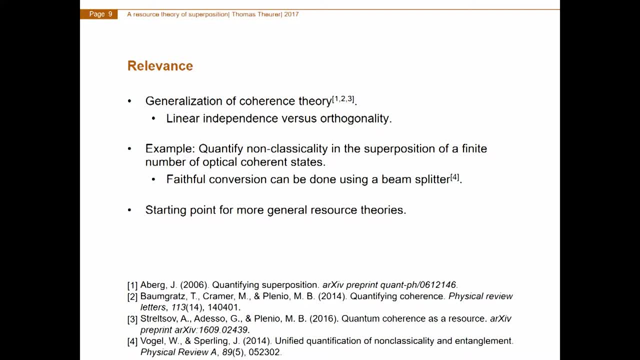 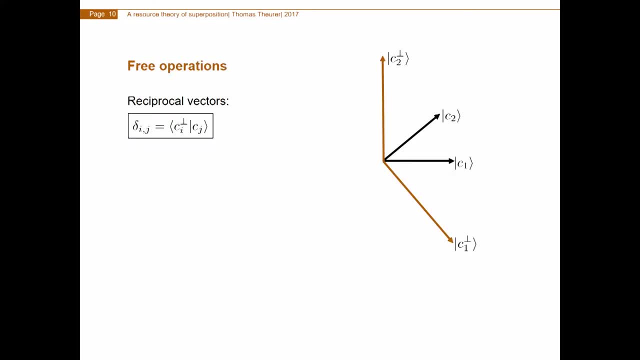 And maybe most important, this resource theory here can be seen as a starting point for more general resource theories, and I will comment on this later. Okay, I hope I have motivated the work. Now we have defined the three operations. We are the three cross operators. 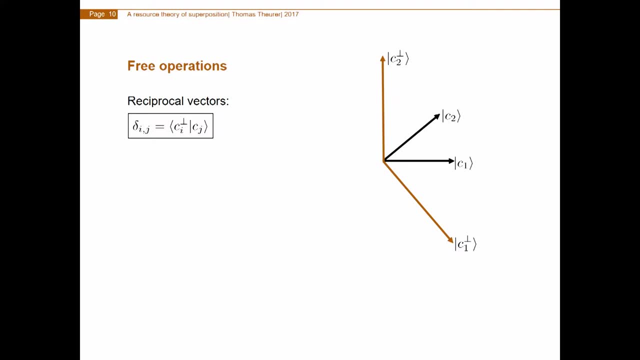 and we would like to characterize them explicitly. In order to do this, we can use the method or the idea of reciprocal states or vectors which you might know from unambiguous state discrimination. So these are just, since our set of free states is linearly independent. 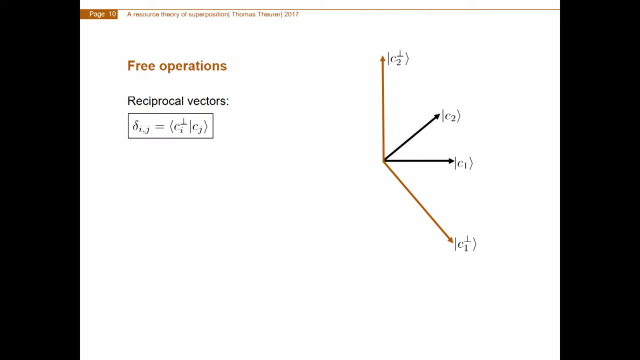 we can always define another set of states which are orthogonal to all states but to one. So in 2D real space we have our two free states and then we can always find states like this. So C1 orthogonal is orthogonal to C2. 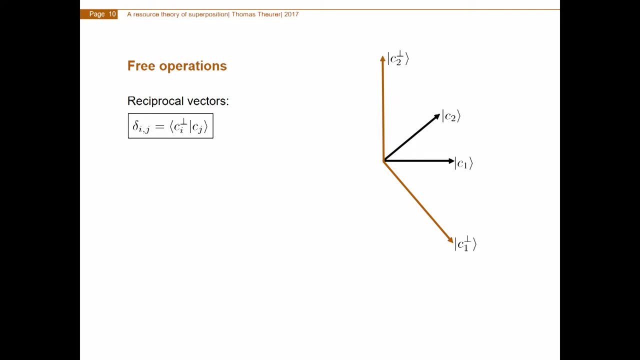 and its projection onto C1 is one. So they are not really states, but rather vectors, because they are not normalized. Now, if we have these vectors at hand, we can write down the explicit form of the three cross operators. So these are all cross operators that have this form. 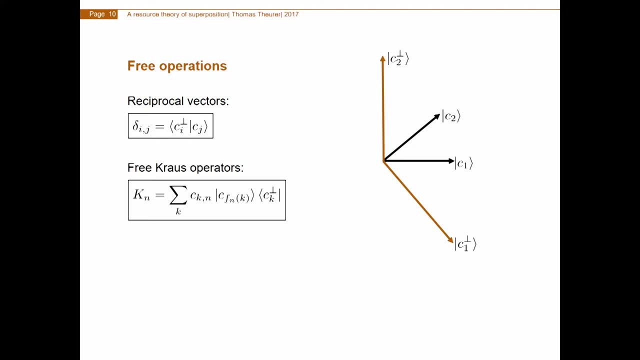 where the Fn of k- this is just a function that gives me an index- and the Ck and their complex valued coefficients. Now, another question which is very important if one deals with trace decreasing or trace non-preserving quantum operations, is whether we can complete a map. 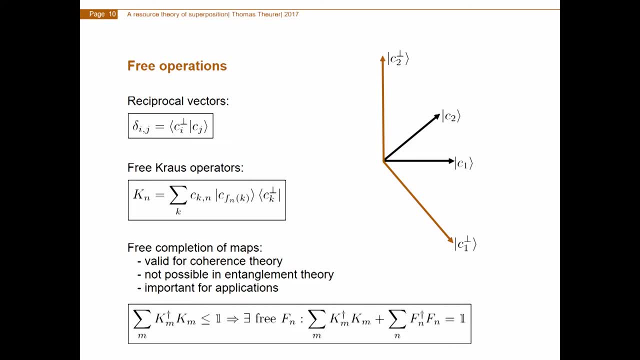 which is trace decreasing for free. So, for example, if we have a map that we can decompose into three cross operators but which is not trace preserving, then we should naturally ask ourselves: well, if we want to implement it physically, we always have an operation. 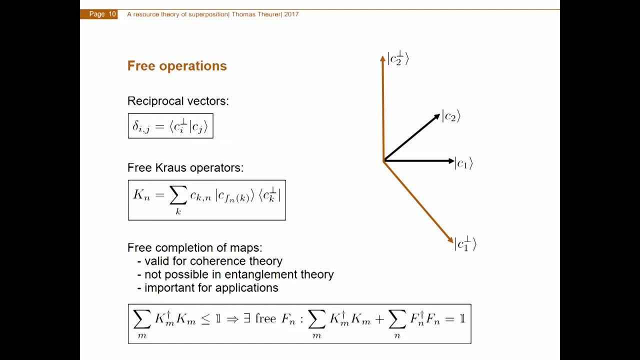 which is in total trace preserving, And if we cannot implement the missing part for free, then we shouldn't really call it free, because it's just then neglecting the part in which we do something non-free, which we cannot do in a lab. So 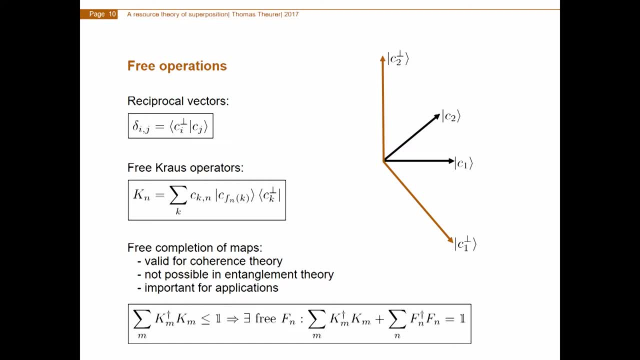 this last statement is very close to the question. No, it's not valid for every resource theory. So in this theory here we can whatever trace decreasing map. so it doesn't even have to be decomposable into three cross operators. we can find three cross operators that complete it for free. 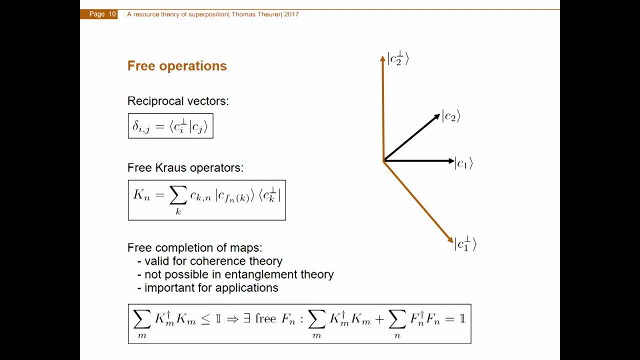 But in entanglement theory that's not possible because there's the problem of uncompletable matrix product basis, so that's not possible in general. Here it is And, as I already said, that's important if you want to work on it. 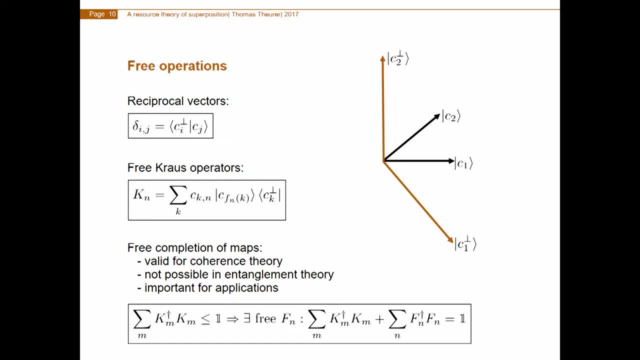 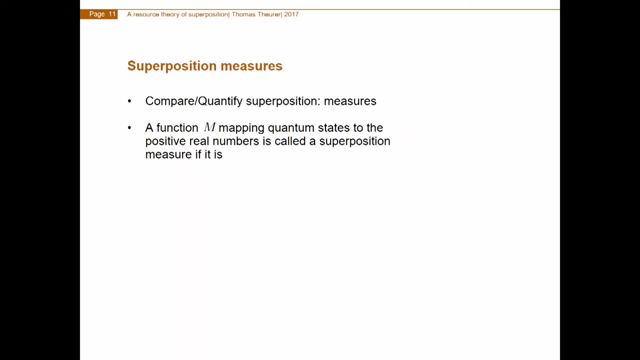 You want to work with trace decreasing operations, And it was also an open question in coherence theory. but since coherence theory is basically a special case of this theory, where your free states are orthogonal, then that's also valid there. Now, if we want to compare the superposition in different states, 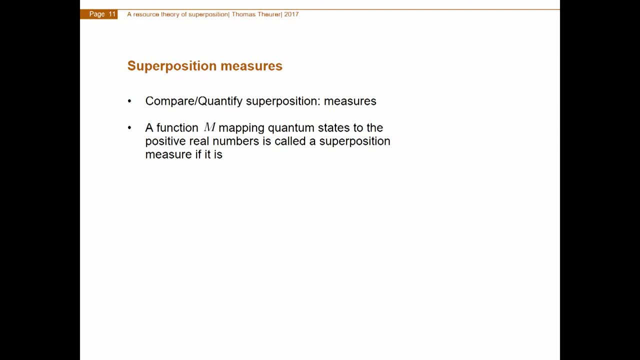 we want to put a number on them and say: well, if the number for associated one state is higher than the number associated with another state, we have more superposition. And, as in other resource theory, we do this by so-called measures. 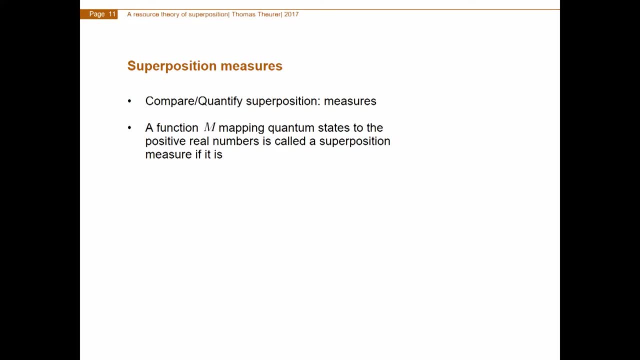 So this is a function that maps quantum states to the positive real numbers and it's a measure if it satisfies certain axioms on which you can also argue, and I will present you one set of axioms, which is motivated physically, as it should always be. 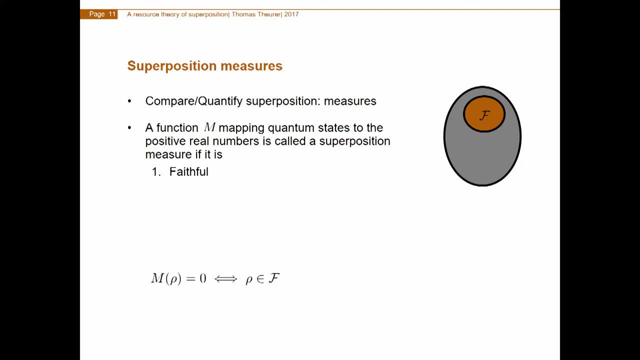 So the first axiom is that it should be faithful. So the measure should be zero on all free states and it should be non-zero on non-free states. So this is really. we have separated our state space into two parts. 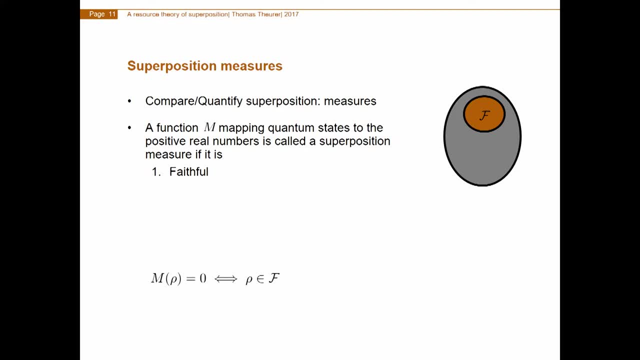 and now we want basically our measure to represent the separation. Then the second property is that our well, as we heard in entanglement theory, our measure should be monotonic under the free operations. So if we take a state, 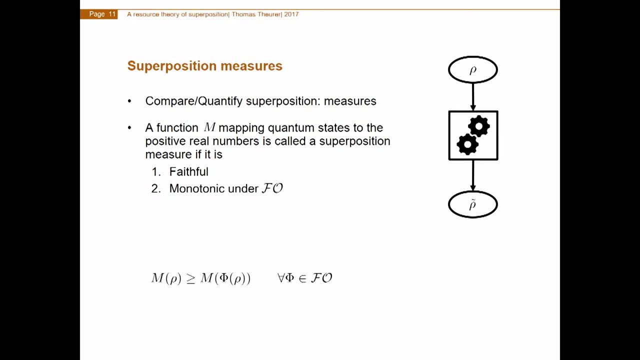 act with a free operation on it, then the amount of resource in the output should be at least- well, it shouldn't be. it should be larger or equal to the amount of resource in the input state. Now the case of monotonicity. 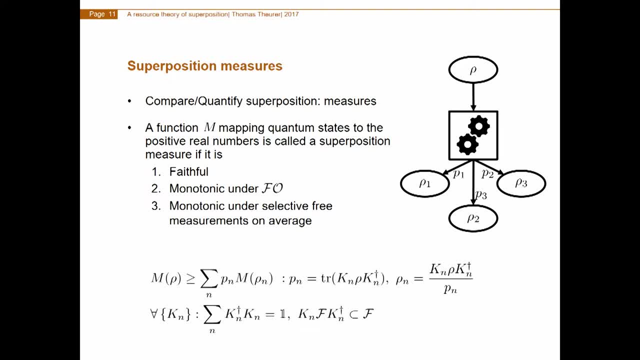 under selective free measurements on average is basically, we do a free operation, we do a sub-selection according to the outcomes and then on average we shouldn't be allowed to use the input state. So if we take a state, we should be allowed to use this method. 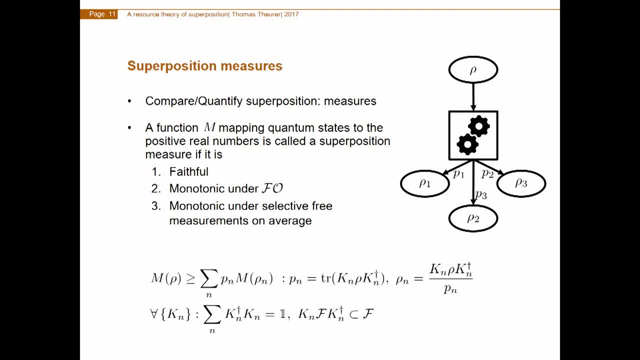 to increase the amount of resource we have. And the fourth condition, which is convexity, basically states, if we mix two states, we do not want to use this to be able to use this procedure to create resource states. Now, if we have properties, three and four together, 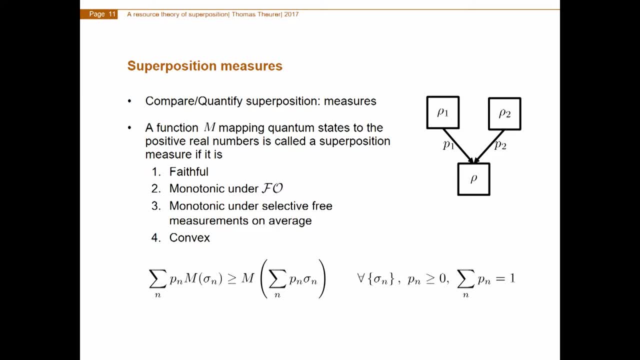 this implies property two, and there are useful measures or functions that only satisfy some of these properties and they for specific applications. they might be useful as well. so that's why I've kept this point two of monotonicity under the free operations. 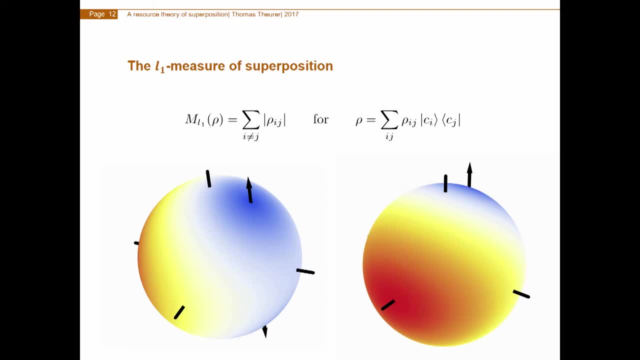 One measure that satisfies all these axioms is what we call the L1 measure of superposition. and if we have a quantum state, we can always decompose it into its free bases. Since they are linear, independent, but form a basis, such a decomposition is always possible. 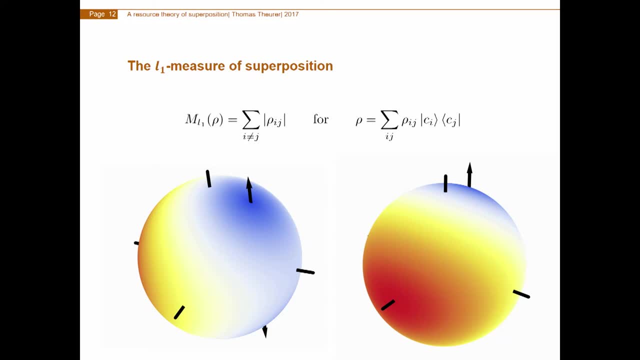 And if we then add up the absolute value of all kind of off-diagonal elements, then this is a function that satisfies all four axioms I've presented to you before, And the advantage of this measure is that it has a closed form. So there are other measures. 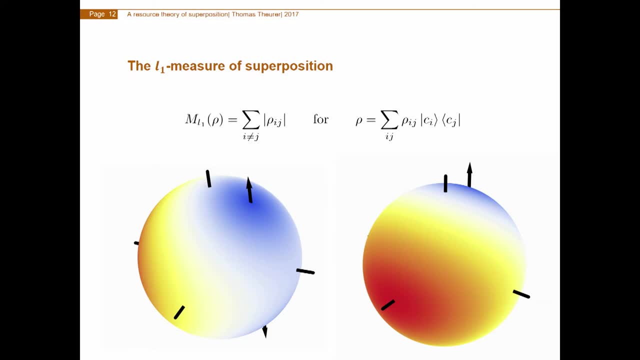 but usually they include some minimization. some maximization And since this is closed, we can calculate it for qubits explicitly. So if we have the free form, we have three states which are depicted by this line of the arrow. 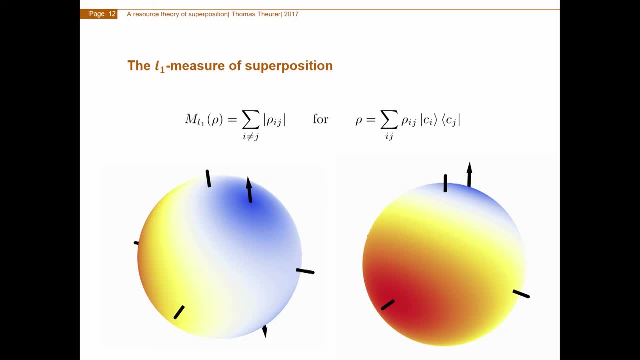 then the L1 measure is low in the blue area and high in the red area. So the further we go away from these three states, the more superposition we have As an all-resource theory. an important question is if we have one resource state. 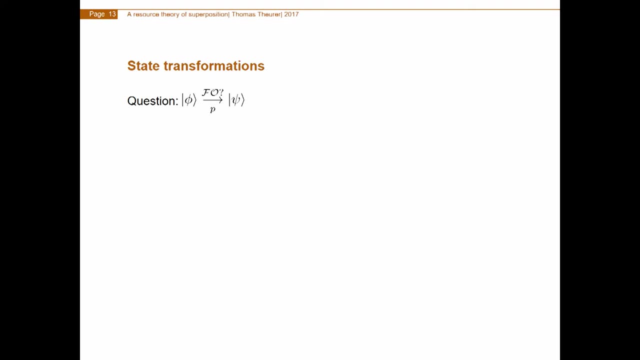 and we use only the free operations. can we transform the state into another resource state or, in general, into another state? Can we do this deterministically? or, if not, can we do it at least with a probability p? And if yes, 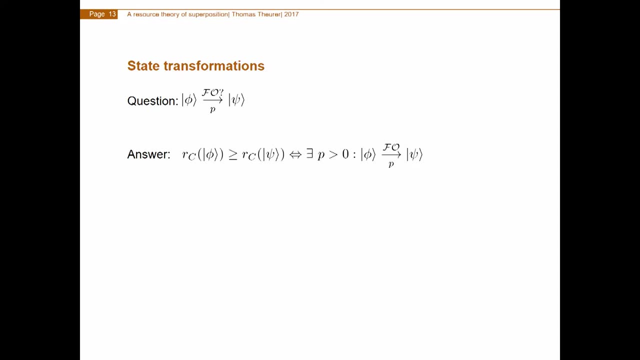 what's the highest probability to do so? Now, the first question is: okay, when are probabilistic transformations possible at all? And the answer is in this classical rank. so the number of states we need to bring into a superposition of three states. 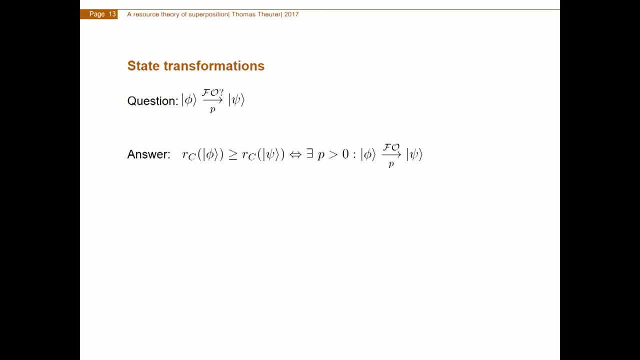 And whenever the classical rank of the initial state is larger or equal than the classical rank of the final state, then at least a probabilistic transformation is possible, And if not, then the probability is strictly zero. Now, if such a probabilistic transformation is possible, 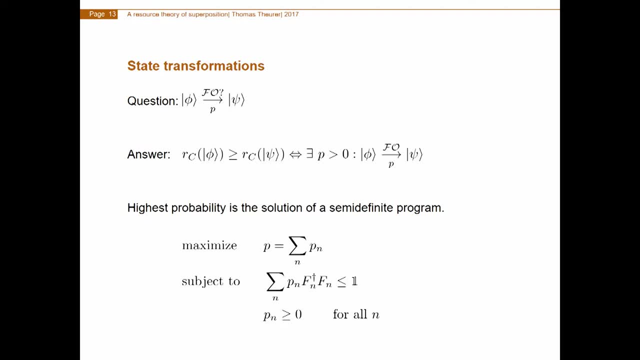 we would like to know well what's the highest probability, p, And the answer to this question is given by the solution of a semi-definite program. so we need to maximize the probability under some constraints, And the Fn is here. these are cross-operators. 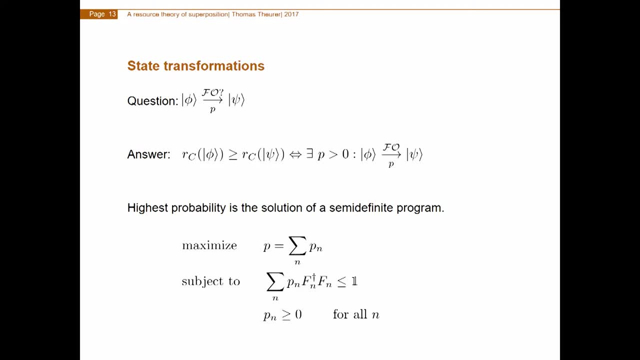 they are known and they depend on the initial and the final state, And using such a description in terms of a semi-definite program is useful, because we know how to attack these problems numerically and there are also loads of analytical results concerning the treatment of these problems. 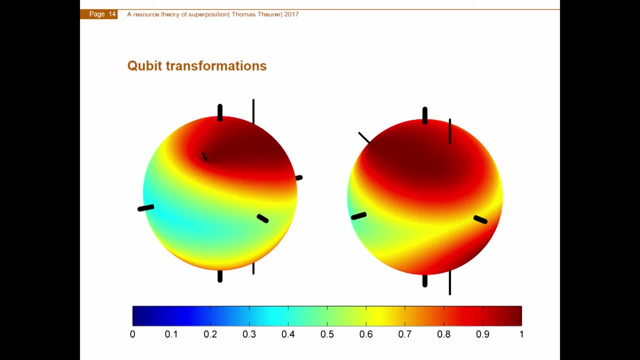 Now for qubits. we have to take into account that, to help with the semi-definite program, we can analyze the maximal probability of transforming one state to another one. Again, we have the three states depicted by this tiny line here. 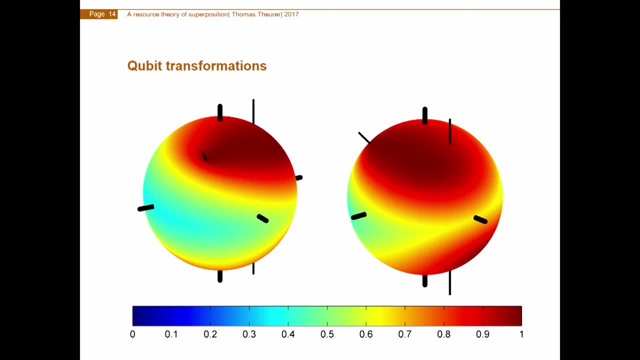 and our initial state is denoted by this line here and here. so it's the same image, just from different points of views. And if we take this initial state, then in this color scheme here on the Bloch sphere is encoded the maximum probability of transforming it. 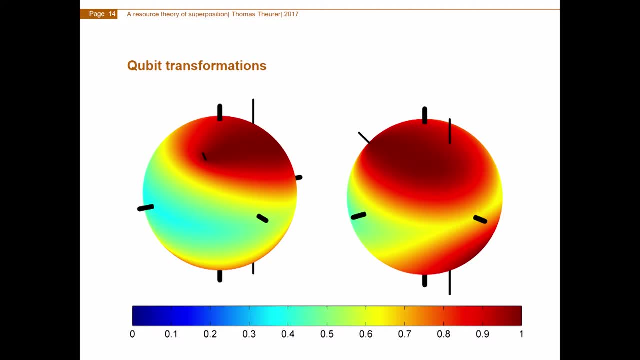 to, for example, this state. it's close to one to this state. here the probability is well about one half And, as you can already see, it's not, at least in the Bloch sphere. it's not really easy to see. 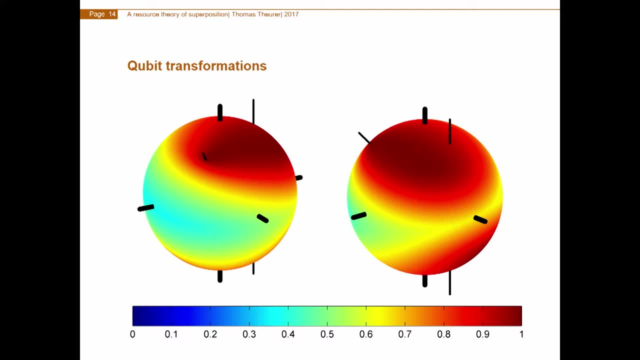 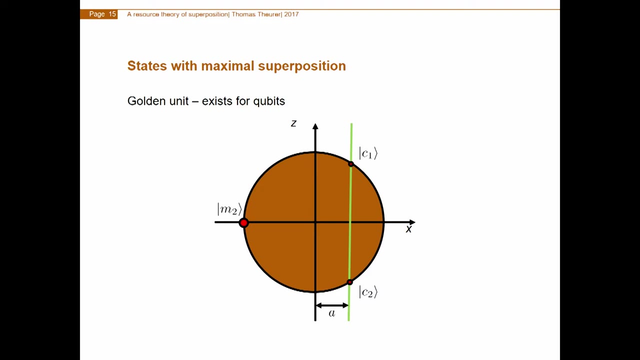 first to which state we can transform it with certainty and then how we can estimate the probability of maximum transformation probability. If we have one state which we can transform with certainty to all other states, then it's the most useful state, so it's the state with maximal superposition. 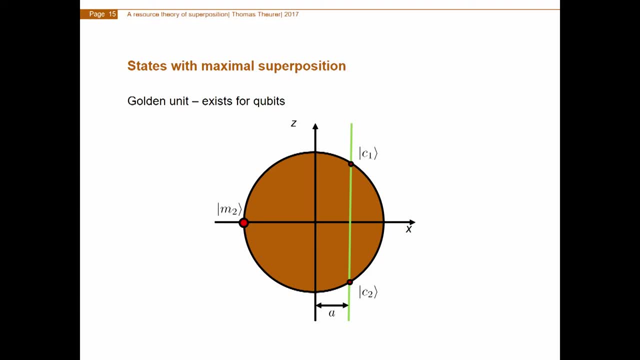 because we can use it for all applications, for all protocols, And so it's often called a golden unit, And in the case of qubits such a state always exists. So if we have again our two pure free states here and here, 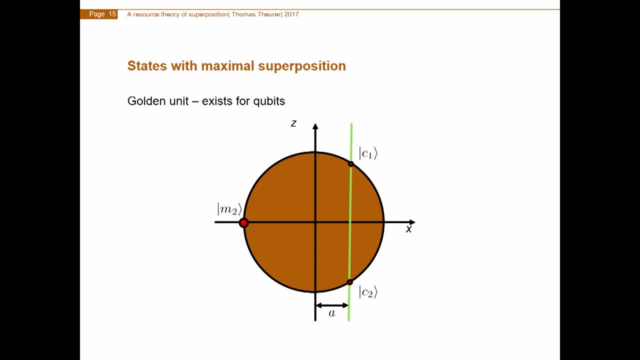 and they overlap A. then the state with maximal superposition is the one on the Bloch sphere, which is the furthest away from the set of free states. So this state, here we can use only free operations and transform it into all other qubit states. 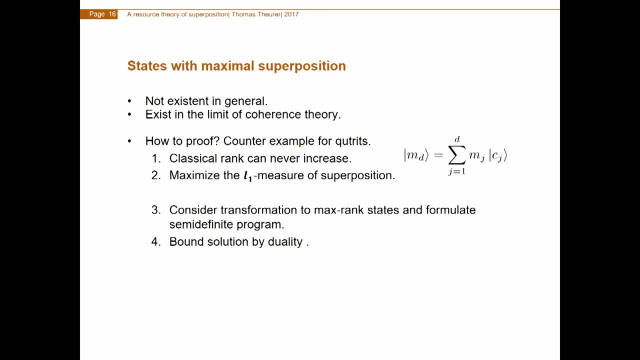 For higher dimensions. this is, in general, not the case In the limit of coherent theory. such states exist, but here not. And now I want to give you a rough idea of how we can prove this, because it basically uses everything I've talked about so far. 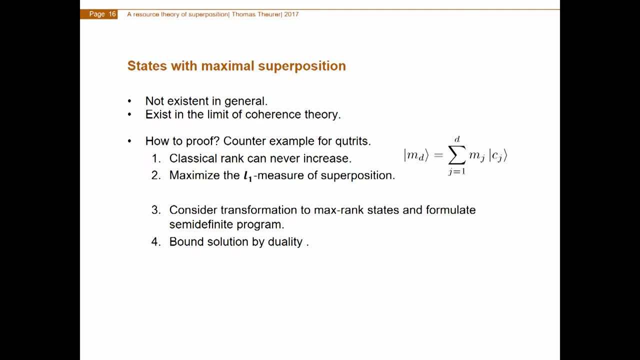 So it exists out of two steps. So first we find certain candidates, so states which might in principle be maximally non, or states with maximal superposition, and then we show that none of these states, indeed, can be used to create all other states with certainty. 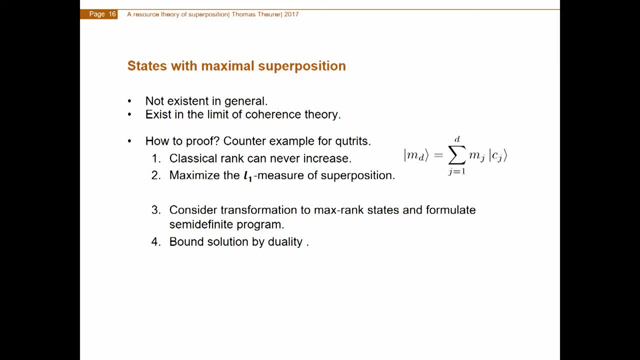 And to do this we just build a count example in 3D. So we choose a basis, a classic basis or three free states, and then we notice: well, if they want to be, if they want to be maximal states. 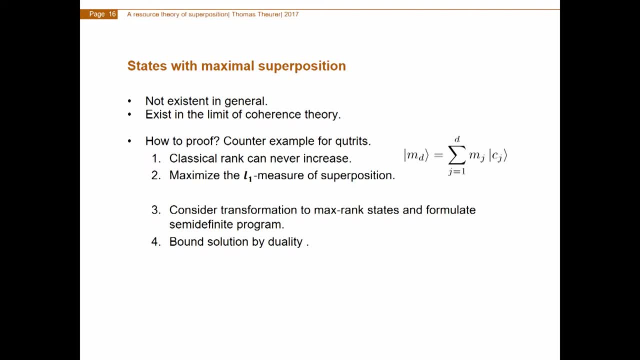 with maximal superposition. they have to maximize all possible measures because they cannot increase under the free operations, And so, in addition, we have already seen that a classical rank can never increase. so we need states that have maximal classical rank, and amongst these states, 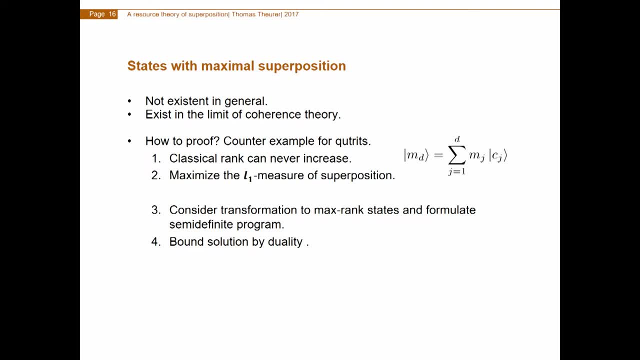 we want the ones which maximize the L1 measure of superposition. And if one chooses the basis with an isometry, one can do this relatively easily, easy analytically, and ends up only with a few candidate states, And then one just uses the semi-definite program. 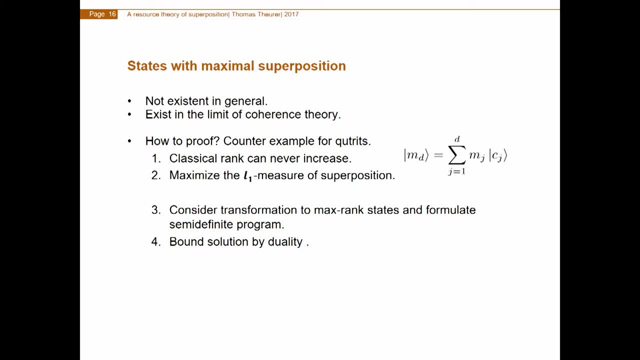 to show that these candidate states, they cannot be transformed to certain other states with certainty. And this can be done analytically because for the semi-definite programs we have the property of duality, so we can transform them into another problem. 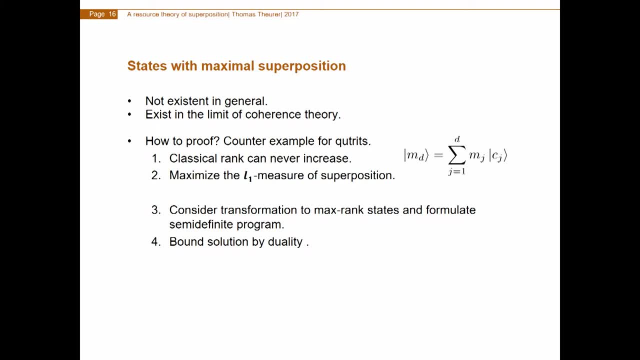 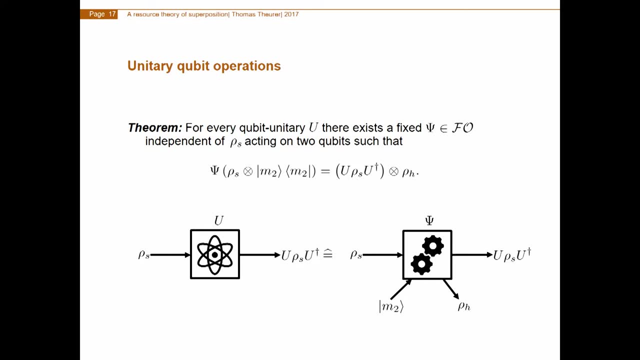 bound to solution of this problem, and then we have also bound on the initial problem. Okay, now, if we have this resource, what can we do with it? So, does access to the resource really grant us with an additional power or with additional possibilities? 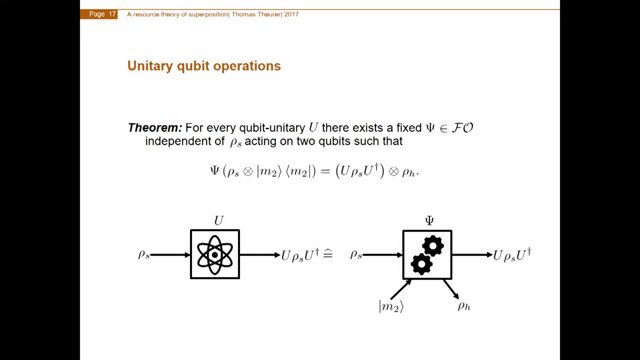 And indeed, if we have access to the resource, we can overcome the restriction. So if we have a unitary, an arbitrary unitary that acts on qubits for simplicity, then well, we have. for every input state, we act on it like a unitary. 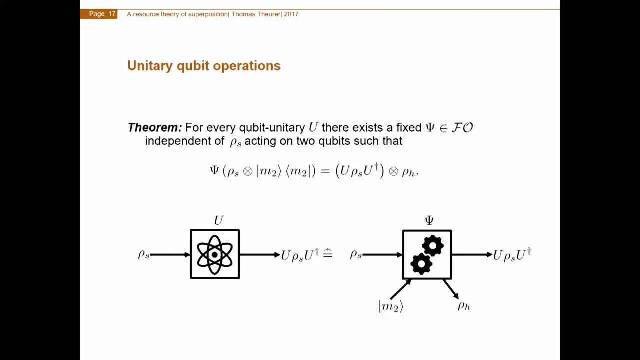 a qubit unitary and this is basically equivalent, or we can reproduce this operation using only a free operation, psi. that acts on two qubits And what it does? it acts on the target qubit on which we want to apply the unitary. 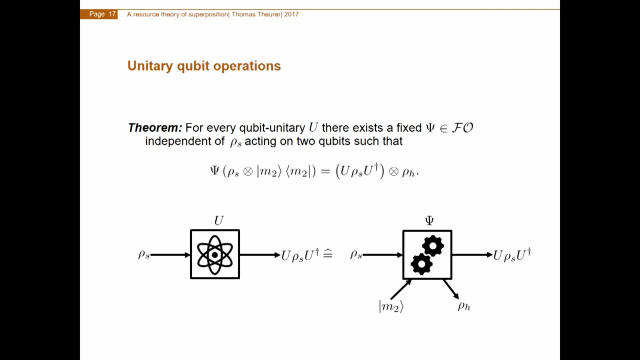 and in addition it acts on another qubit state which is in a maximum superposition state And the output is separable. and we have applied the unitary on our target qubit and we have basically destroyed the superposition in our auxiliary qubit. 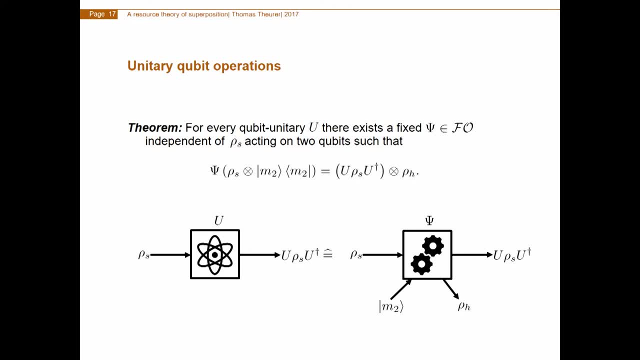 So we have used the resource, we have consumed it in order to overcome the restriction, And it's maybe important to emphasize that for a given unitary, this psi here is independent of the input state. So it's really we reproduce the operation. 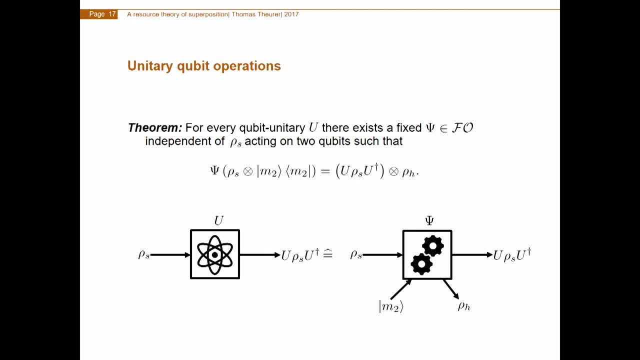 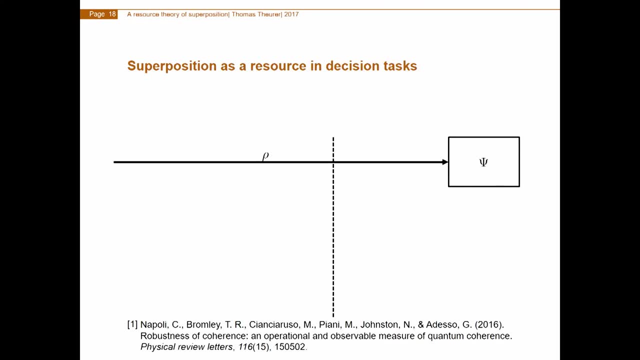 and we do not only reproduce the action of the operation on a certain state. In addition, we can use superposition as a resource in decision tasks. So decision tasks are, as we heard yesterday, a part of quantum metrology, And we can well basically describe it. 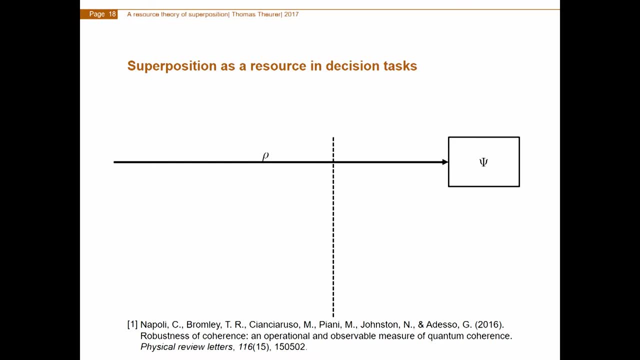 as a quantum game, And something similar has been done in the case of coherence in this paper. So we have two players: Alice and Bob. Alice might or is allowed to say or is allowed to send a quantum state to Bob, who applies a quantum operation on this state? 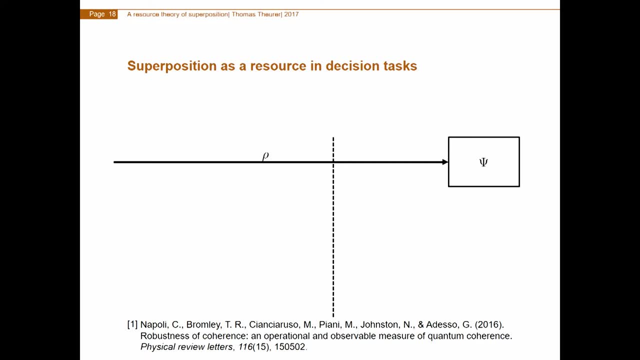 And this operation is a selective measurement with d plus one outputs. If the output is zero, then he just says: well, please give me another state. So he asks for a new term. However, if the output is not zero, he returns the output state. 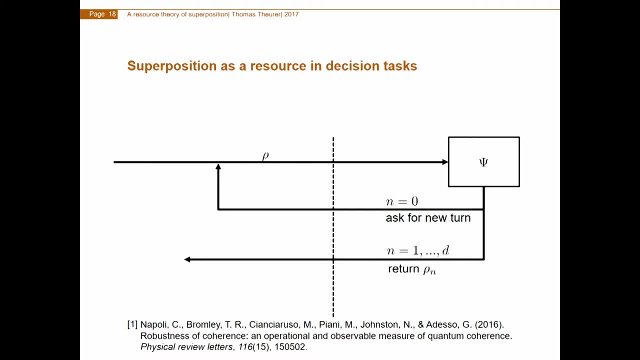 of his quantum operation to Alice. Now, the goal of Alice is to get Alice, so she wants to find out, basically decide which output n Bob received And in order to do this, she's allowed to do an arbitrary quantum operation on this state. 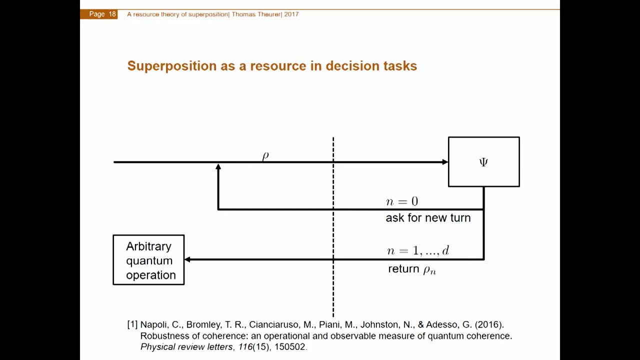 Now she has two possibilities. For example, she might do unambiguous state discrimination in order to find out which n Bob obtained. Well, if this fails, then she has the ability to just ask for a new term, So she can hand in a new term. 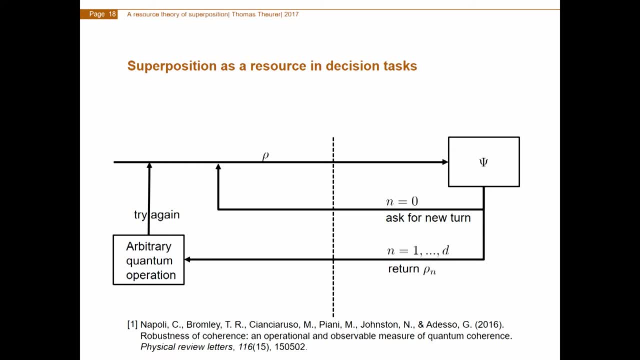 so she can hand in another state, a new state and try again. However, she can also make a guess, And if she's correct she wins, If she's wrong, she loses. Now, if we use a certain quantum operation here, 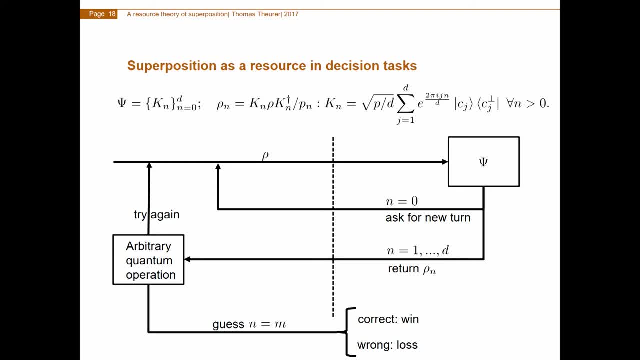 so a free quantum operation then, for n not equal zero. what the operation does is it basically imprints a phase which is dependent on n, which is dependent on free states In the case of n equal to zero. this failed and Bob asks for a new term. 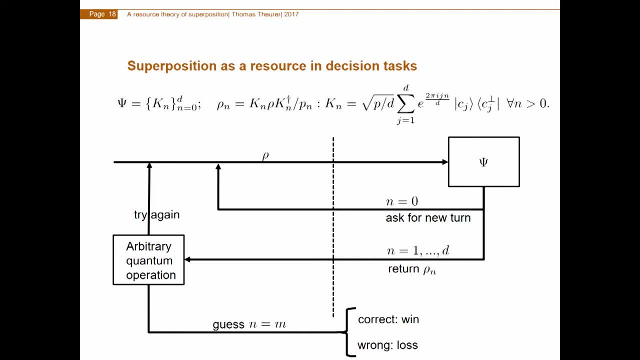 Now, if Alice has only access to free states here, then she cannot win the game in the limit of large D, because the output row n is independent of n. So whatever free state Alice puts in row n is the same for all n. 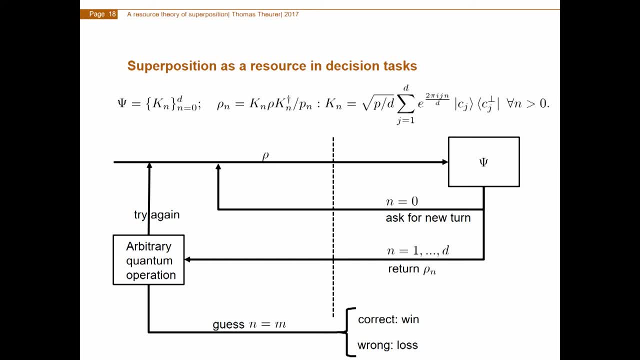 And if well, in the limit of large D we have. and, in addition, the probability of output n is the same for all n. So the best thing Alice can do is make a random guess and if well, if you have. 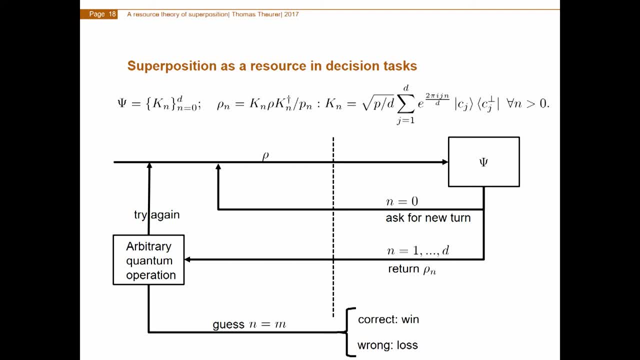 a high enough dimensional Hilbert space, the probability of making the right guess goes to zero. However, if she has access to certain superposition states, these output states are different and, in addition, they are linear independent, so she can do indeed. 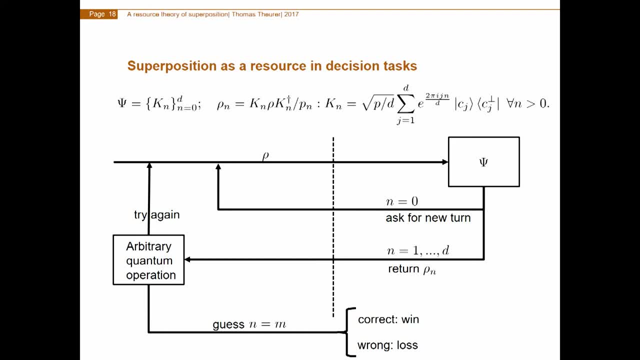 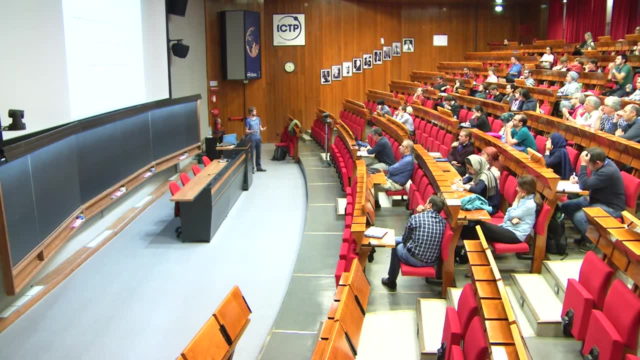 state discrimination when it fails. so when she gets an indecisive answer, she just tries again. and if she gets a decisive answer, well, she can guess with certainty, so she can give the correct answer for sure and thus win the game. 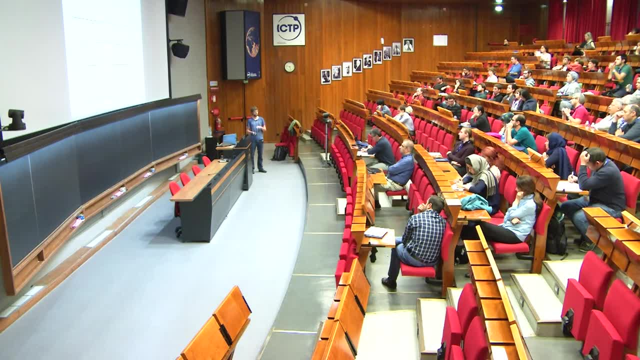 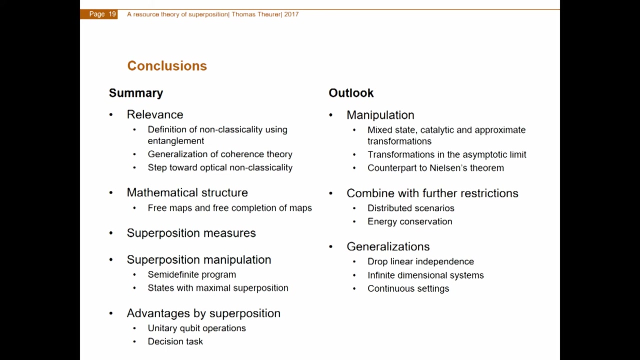 So access to the superposition states basically turns certain loss into certain win. Sorry, Okay, Now let me come to my conclusions. So I hope I have convinced you about the relevance of this resource theory so we can use it to define the a bit vague definition. 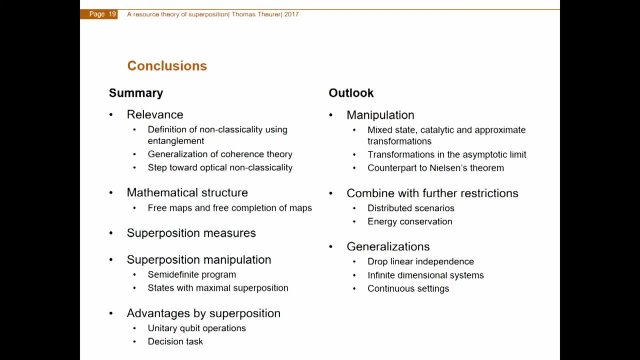 of non-classicality using entanglement, Then it's a generalization of coherence theory and, most importantly, it's a step towards quantification of optical non-classicality. So we've spoken a bit about the mathematical structures, for example, of the free maps. 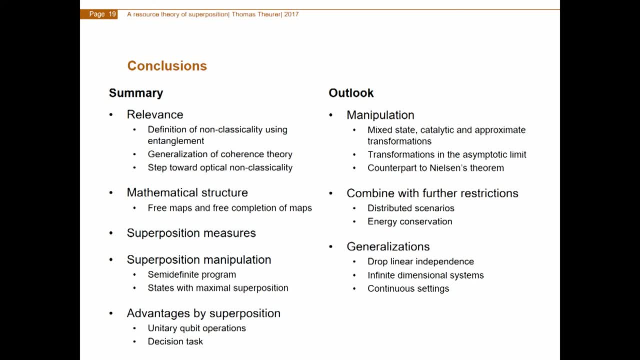 and the completion of free maps. I've introduced to you the concept of superposition measures and we've spoken about superposition manipulation in the form of a semi-definite program, and we've investigated states with maximum superposition And we also noticed. 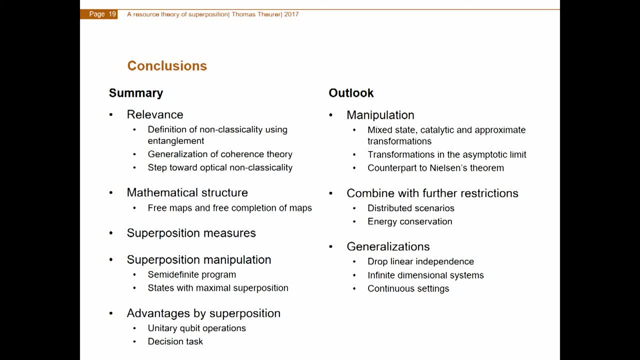 that there are advantages in superposition, in having access to superposition states. Now, of course, that's far from being completed, the theory. so we haven't said anything about mixed state transformations, And what is also a very interesting concept is the concept of approximate transformations. 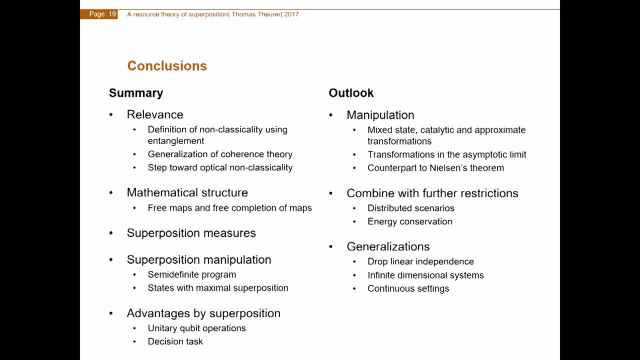 So we want to transform an initial state not exactly to a target state, but only approximately to this target state. Also, we have only considered transformations in the asymptotic limit. No, we have not considered transformations in the asymptotic limit, so we have only focused. 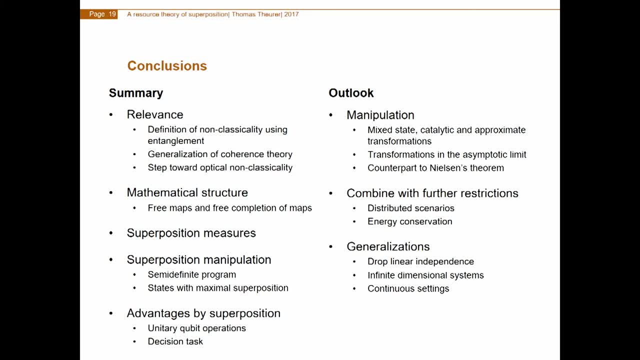 on single-copy transformations. So I have only one copy of the initial state and not access to other copies. Well, and all these state transformations. it would be very nice to find a closed condition when we can transform one pure state into another pure state with certainty. 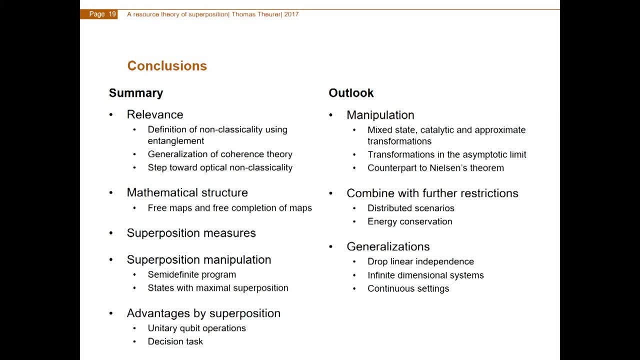 Because at the moment there's still a solution of a semi-definite program which you have to solve. Well, as in other resource theories, especially in the resource theory of coherence, we can combine this restriction with further restrictions, So one can think about. 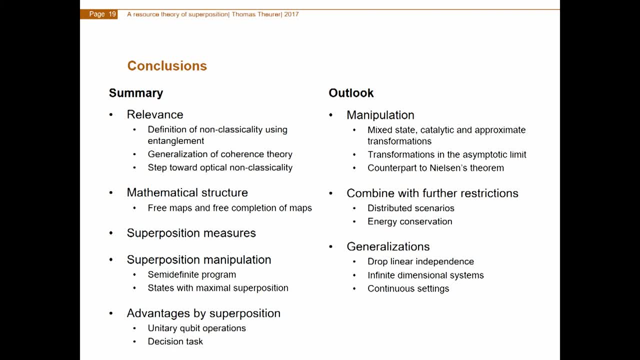 local superposition-free operations. So, for example, if I have some spatially separated labs, I should in a sense include the idea of spatial separation and of classical operations on the systems in the lab itself And for mesoscopic or macroscopic systems. 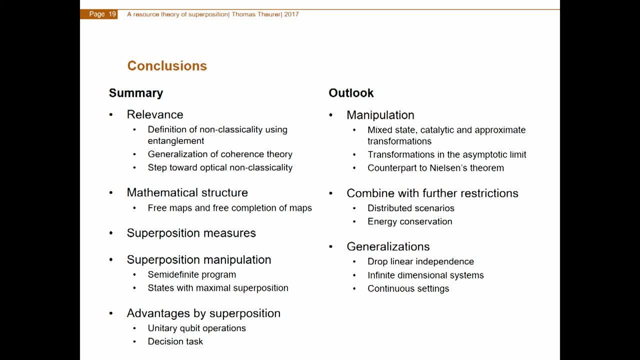 one would also like to include energy conservation, for example. But the most important next step, in my opinion, is that one works on generalizations of the theory. So it's still very restricted because we have linear independence. we are in finer dimensional systems. 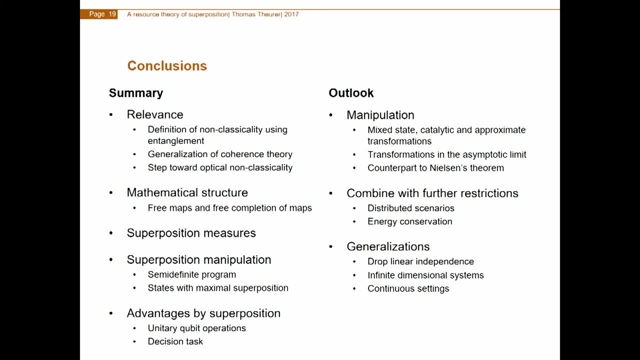 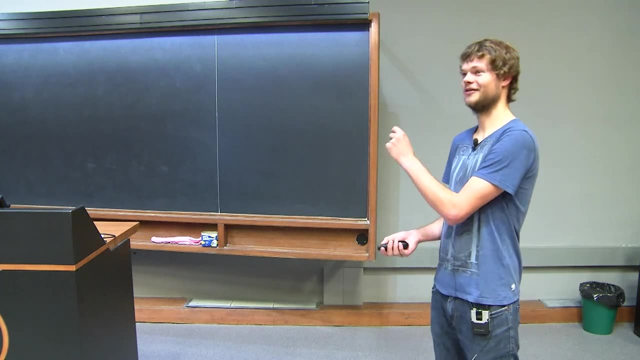 and if one would like to quantify optical non-classicality then one has to go to infinite dimensional Hilbert space. Probably one would like to choose for the free states, the global coherence states, because they are most classical And they are continuous, so they are not only not linear independence.